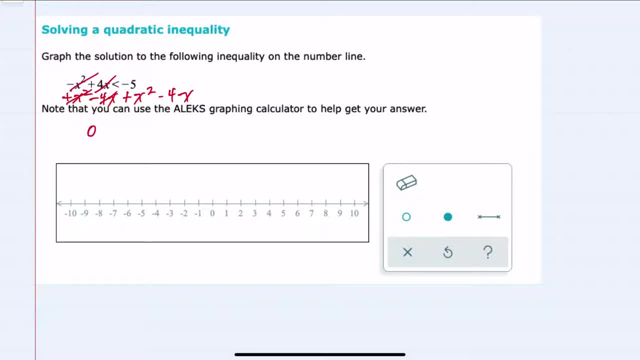 would cancel, leaving me zero. I've only been adding and subtracting, so the direction of that inequality stays the same. On the right hand side, if I were to put all of these in descending order, I have x squared minus 4x minus 5.. From here I have my quadratic on one side. 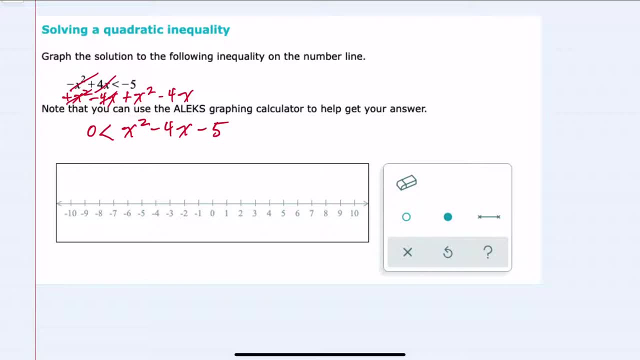 0.. on the other, I would first look for where that quadratic equals zero, and I can find this by factoring the left-hand side. It factors by trial and error with an x and an x. The factors of a minus 5 would have to be 5 and 1, and I'll make the 5 negative and the 1 positive to give me a. 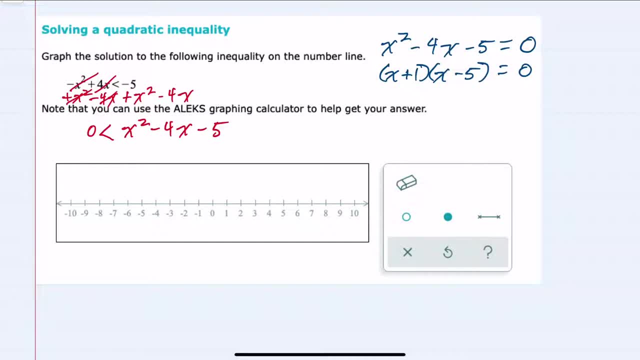 negative 4x in the middle, and now that I have two factors being multiplied to equal 0, I know that either the first one- x plus 1, would have to be 0. This happens when x equals negative 1, or the 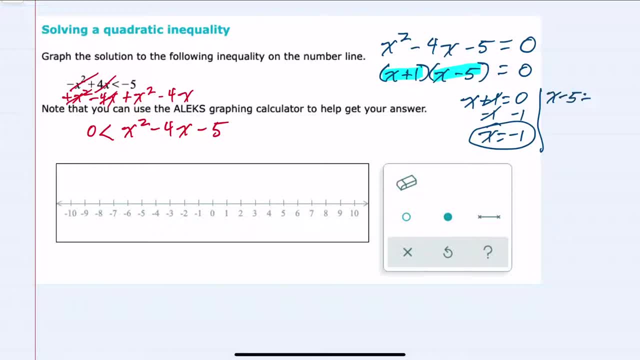 second factor, x minus 5, would have to be 0, and this happens when x equals a positive 5.. So our two points here are negative 1 and 5.. I'm going to look at what happens to each one of these functions, to the 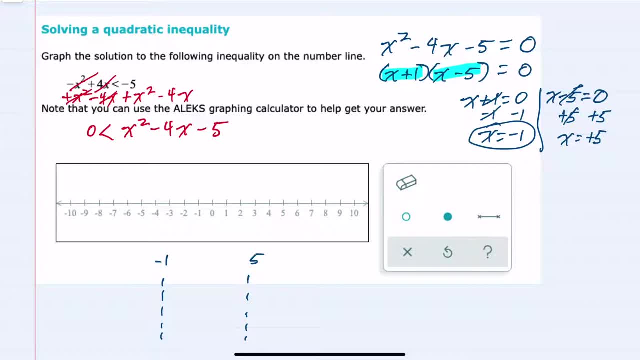 left of negative 1, between those two values and to the right. Starting with our first factor, x plus 1, would be negative if I plugged in any values less than negative 1, and it would be positive for any values greater. Looking at the second factor, x minus 5,. 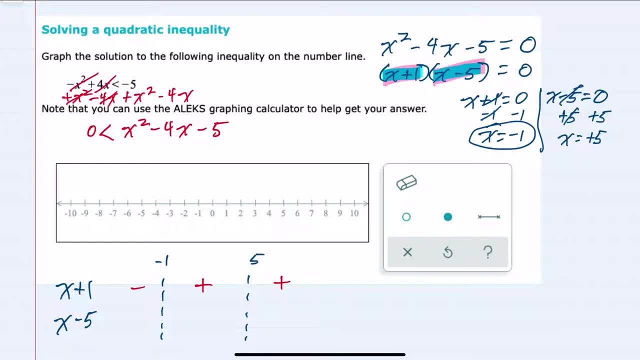 x plus 1, and x plus 1,. I'm going to look at what happens to each one of these functions: x minus 5, any value that I substitute greater than 5 would be positive and any value less than 5 would be negative. and now that I've broken down where each one of those is positive or negative, 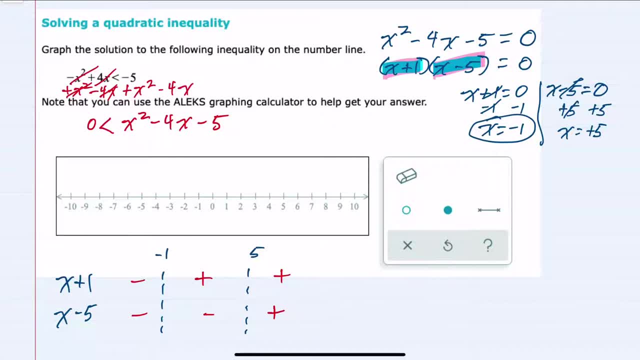 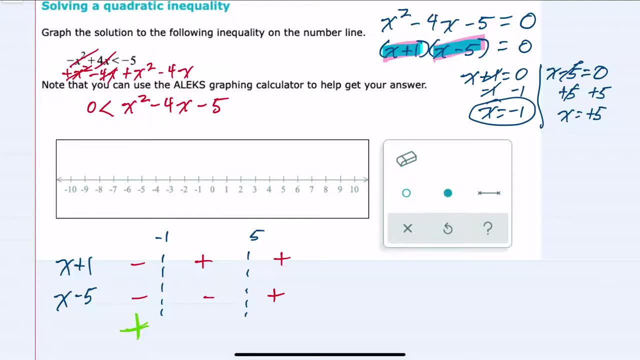 since this inequality has them being multiplied. I can see that to the left of negative 1,, I have a negative times a negative. this would be a positive. Between negative 1 and 5, I would have a positive times a negative, which is negative, and to the right of 5, a positive times a positive is.